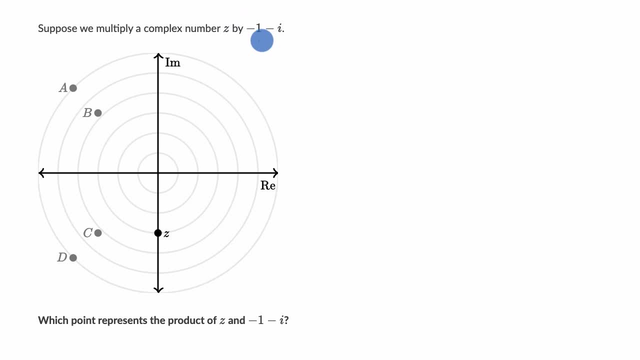 So the way I think about this is: when you multiply by a complex number, you are going to rotate by the argument of that complex number and you're going to scale the modulus of z by the modulus of this complex number. Now let me just think about that a little bit. 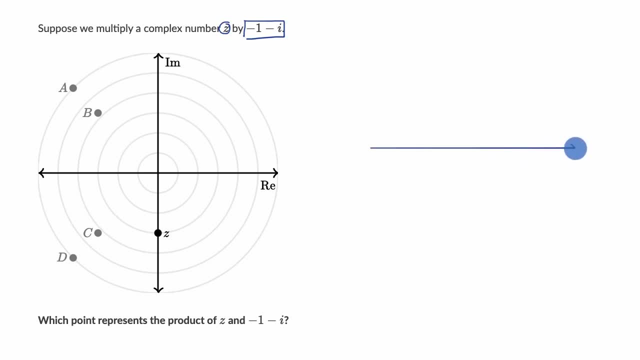 So I'm gonna draw another complex plane here, And so this is my real axis, This is my imaginary axis right over here, And negative one minus i, so that's negative one, and then minus one i, So it would go right over there. 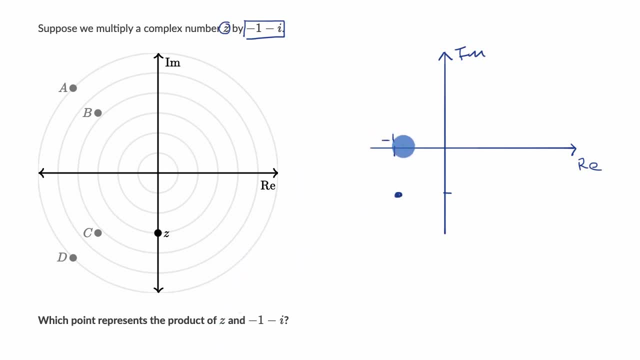 It would be that right over here. And so let's think about two things: Let's think about what its argument is and let's think about what its modulus is. So its argument is going to be this angle, right over here, And you might already recognize. 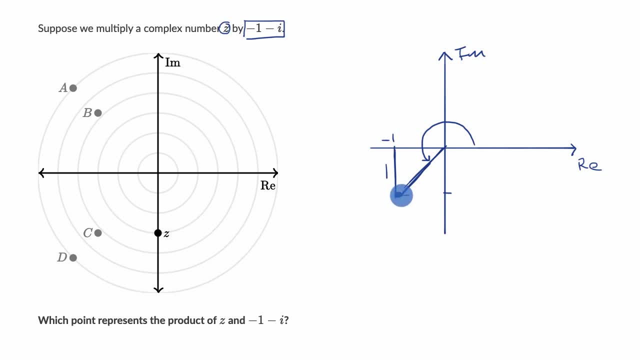 that if this has a length of one, if this has a length of two, if this has a length of three, if this has a length of one or another way of thinking about this has a length of one. this is a 45,, 45, 90 triangle. 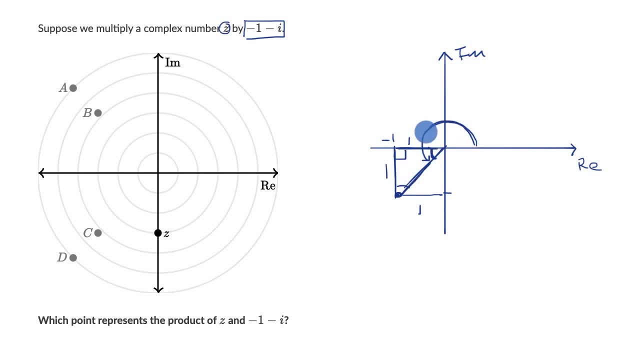 So this is 45 degrees, but then of course you have this 180 before that. So that's going to be 180 plus 45 is a 225 degree argument. So the argument here is going to be equal to 225 degrees. 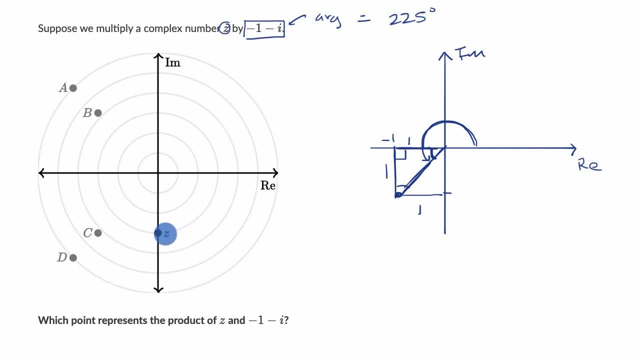 So when you multiply by this, you are going to rotate, rotate by 225 degrees. So let's see, this is going to be rotating by 180 degrees and then another 45. So if you just rotated by that, you would end up right over here. 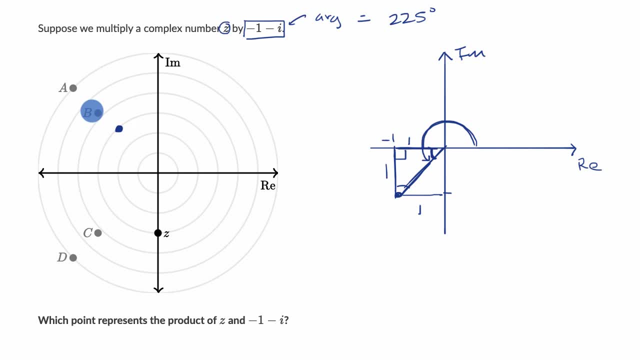 Now we also are going to scale the modulus and you can see two choices that scale that modulus, And so we know it's going to be choice A or choice B, because choice is C or D. you'd have to rotate more to get over there. 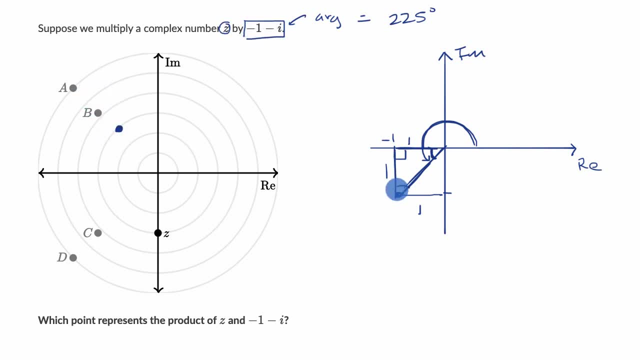 And so to think about that, we have to just think about the modulus of negative one minus I- this point right over here- and then just scale up Z's modulus by that same amount. Well, the modulus is just the distance from zero in the complex plane. 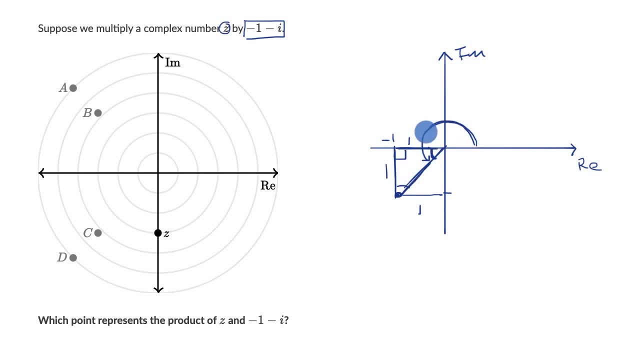 So this is 45 degrees, but then of course you have this 180 before that. So that's going to be 180 plus 45 is a 225 degree argument. So the argument here is going to be equal to 225 degrees. 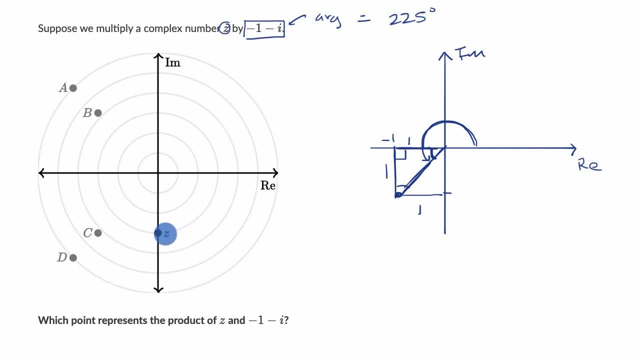 So when you multiply by this, you are going to rotate, rotate by 225 degrees. So let's see, this is going to be rotating by 180 degrees and then another 45. So if you just rotated by that, you would end up right over here. 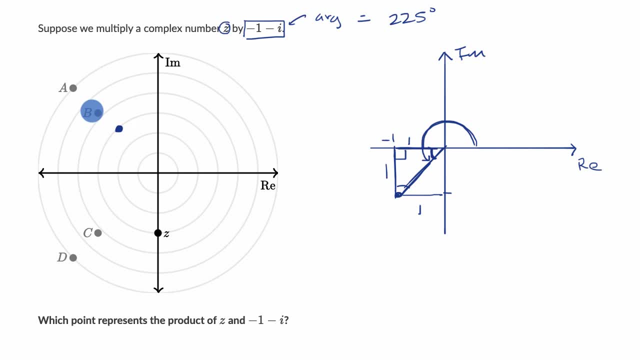 Now we also are going to scale the modulus and you can see two choices that scale that modulus, And so we know it's going to be choice A or choice B, because choice is C or D. you'd have to rotate more to get over there. 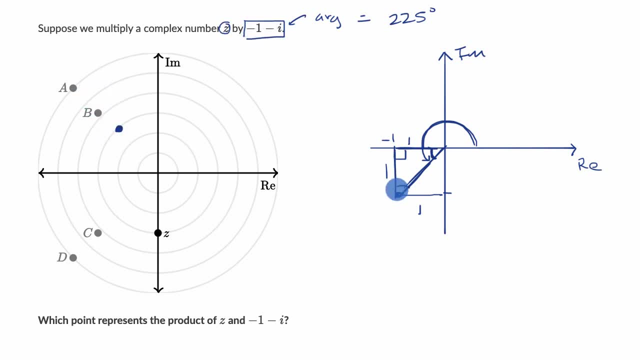 And so to think about that, we have to just think about the modulus of negative one minus I- this point right over here- and then just scale up Z's modulus by that same amount. Well, the modulus is just the distance from zero in the complex plane. 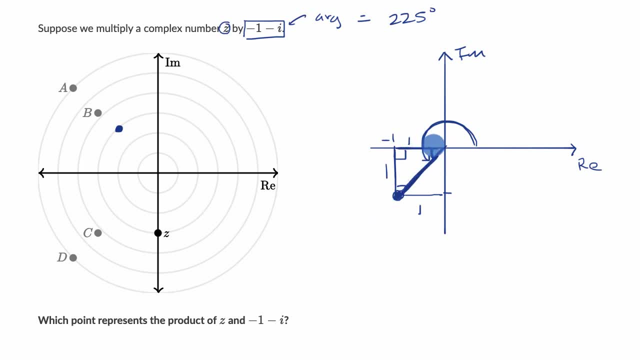 So it's going to be this distance right over here, And you could use the Pythagorean theorem to know that this squared, if you call this C, C squared is equal to one squared plus one squared, or C squared is equal to two. 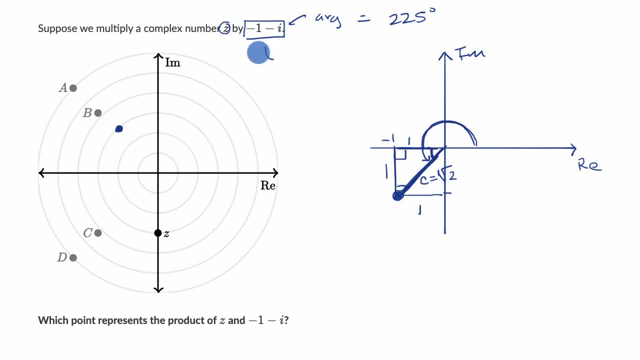 or C is equal to the square root of two. So that's the modulus right over here. Modulus is equal to square root of two, which is approximately. it's a little bit more than 1.4.. So let's just call it approximately 1.4.. 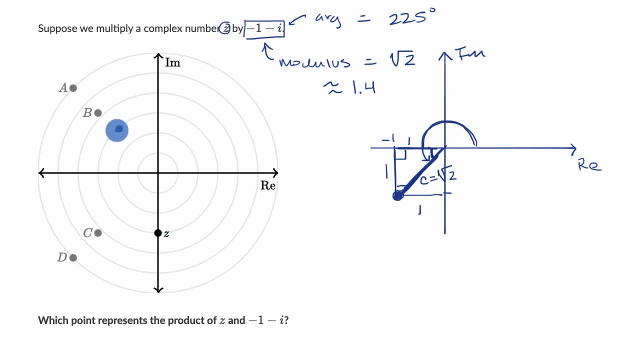 So not only are we going to rotate by 225 degrees, we're going to scale the modulus- the distance from the origin- by 1.4.. So if it is, it looks like it's three units from the origin, right over here. 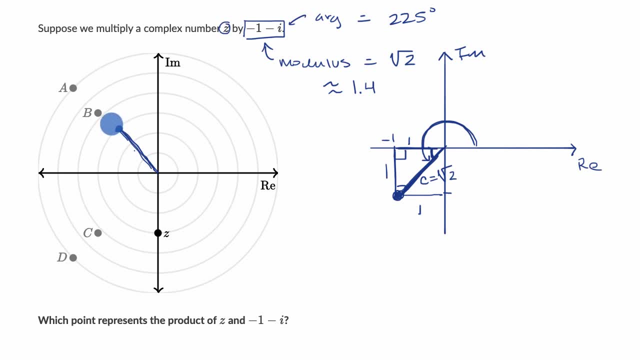 If you multiply that by 1.4, three times 1.4 is about four, or it is exactly four, It's basically 4.2.. So 4.2 of these units is one, two, three, four. 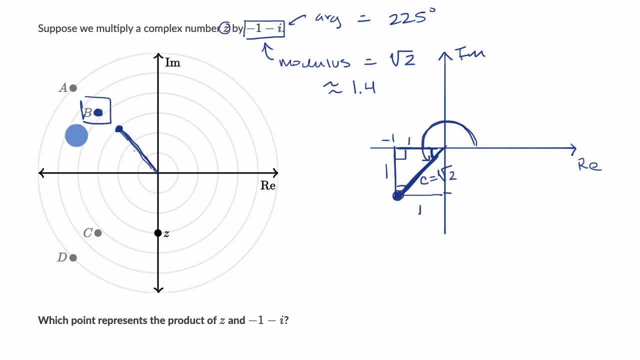 and a little bit further. you get right over here to choice B And we're done. 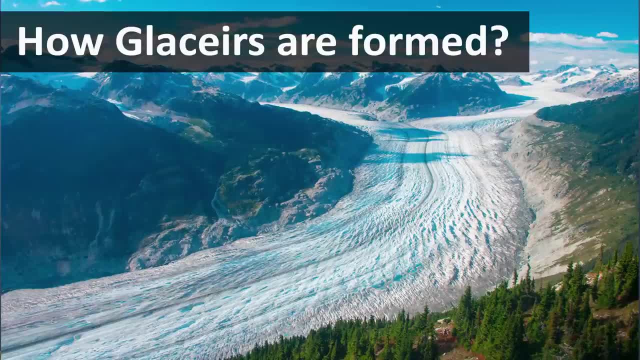 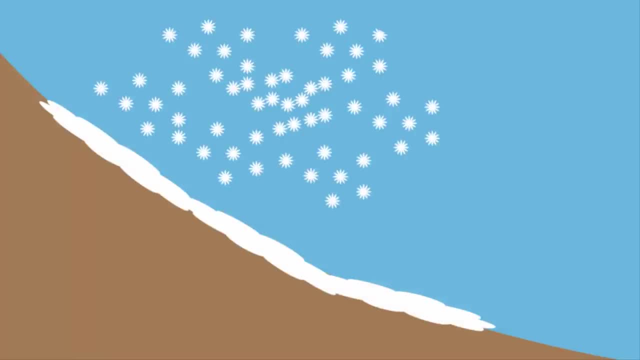 In this video, we will learn how glaciers are formed. Glaciers begin to form when snow remains in the same area for a very long time. I am talking about an entire year. This way, each year, a new layer of snow is formed on previous layers.